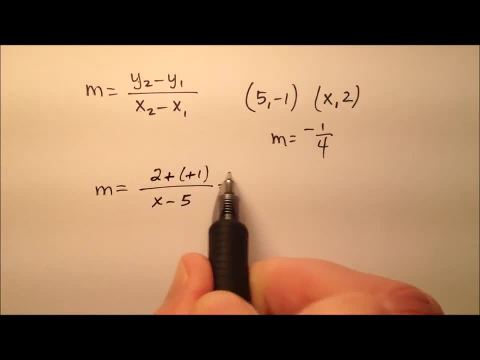 well, let's simplify that a little bit. So 2 minus a negative 1 will give us 2 plus 1, which is 3 over x minus 5.. And now I can set that equal to negative 1. 4th, because I know. 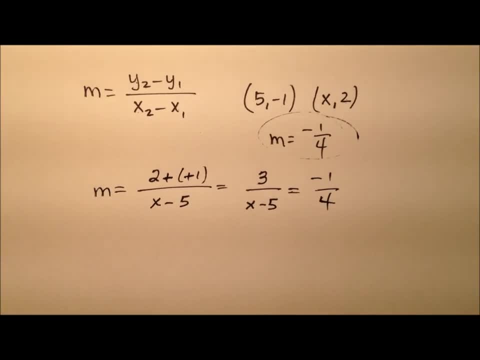 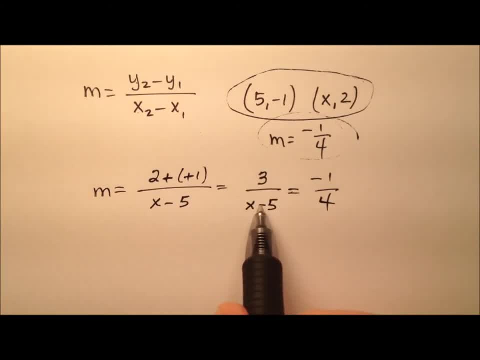 I found out that my slope was 3 over x minus 5, but we don't really know what that x coordinate is. But I do know that my slope is negative 1. 4th, so I can set those two things equal to one another. And now I can solve by using cross products, So 3 times. 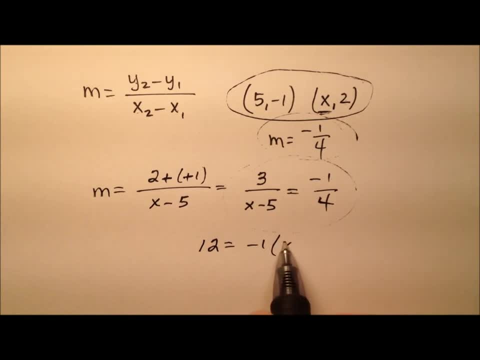 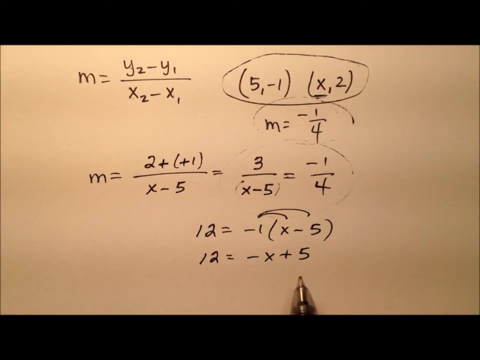 4 is 12, and I'm going to multiply negative 1 times this x minus 5.. And be sure that since this has two terms, we put parentheses around that because I'm going to have to multiply these two terms. So 12 equals negative x plus 5.. So if I subtract 5 from both sides, 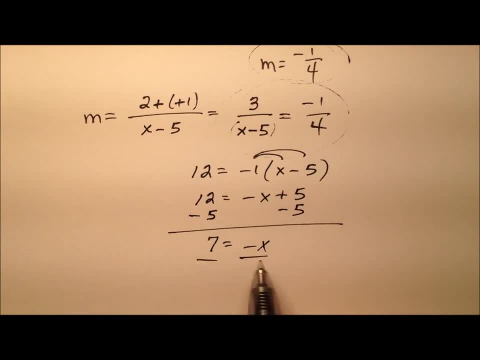 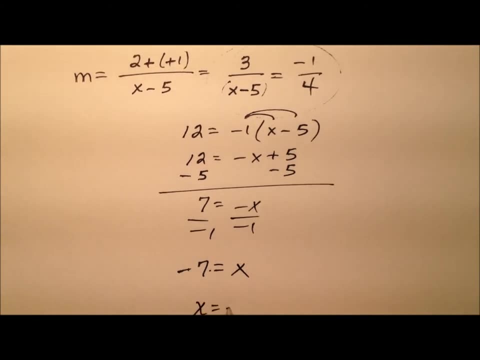 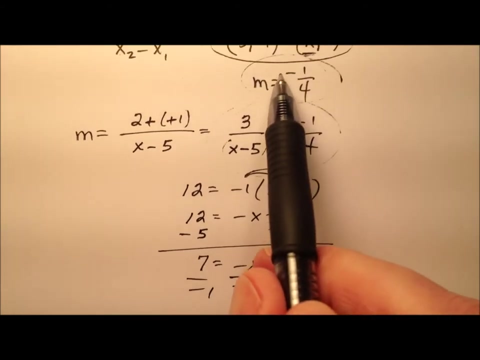 I have: 7 equals negative x. So if 7 equals negative x, when I divide by negative 1, I'll see that negative 7 equals x or, of course, x equals negative 7.. So here is that x coordinate for my ordered pairs. 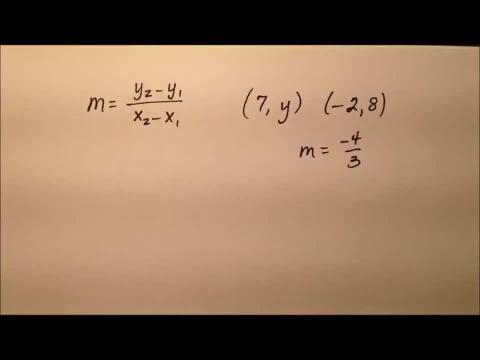 That makes the slope negative 1- 4th. In this second example, once again I have my ordered pairs 7y and negative 2: 8.. Well, it seems like I'm missing my y coordinate in this ordered pair, but I do know that the slope between these two points is negative 4. 3rds. So I 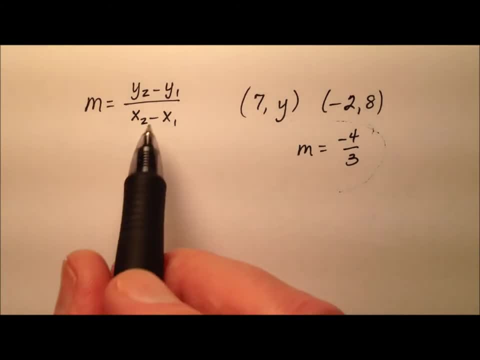 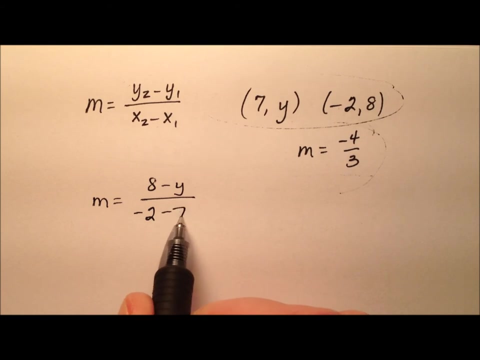 can use that information and find this value of y. So let's go ahead and plug these two ordered pairs into my slope formula, since I know what the slope is. So we're going to say m equals, and then 8 minus y, divided by the change in x, which is negative, 2 minus. 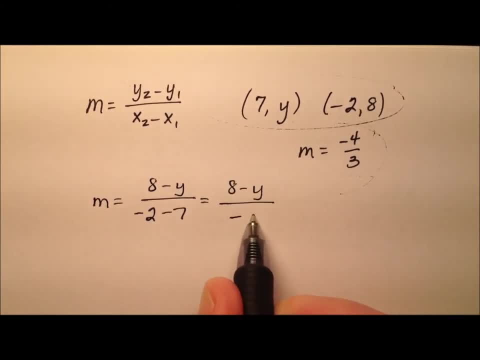 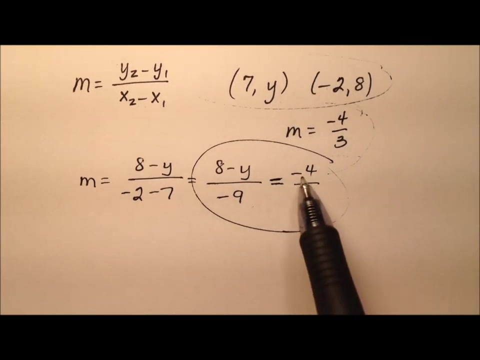 7. So that looks like 8 minus y over negative 9. And this is kind of our simplified form, but we know that equals negative 4 3rds. So I can set up this proportion that says these two fractions are equal to each other, And I can solve by using cross products. So I'm 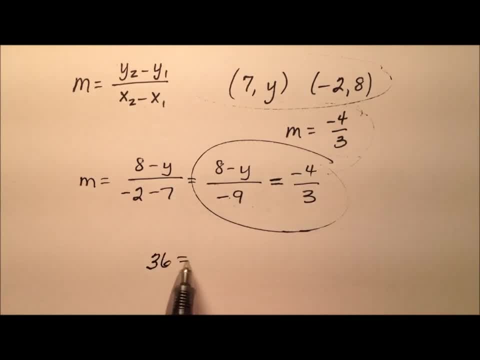 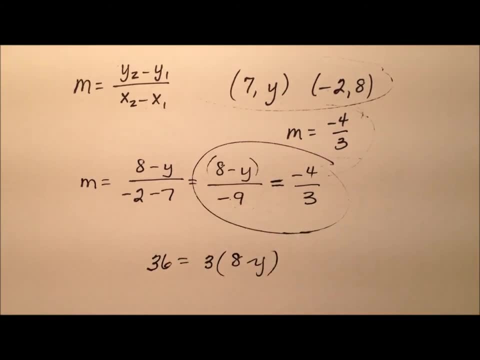 going to say negative 4 times, negative 4, 3rds. So I'm going to say negative 4 times negative. 9 is 36. And that equals 3 times- and I want to put this in parentheses- 8 minus y, because 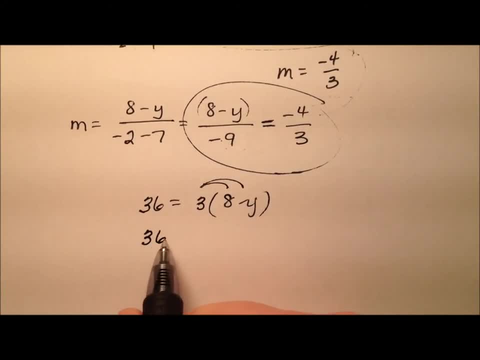 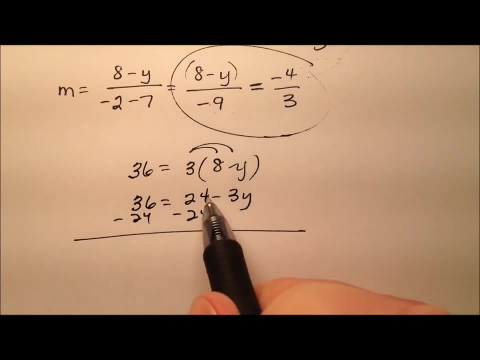 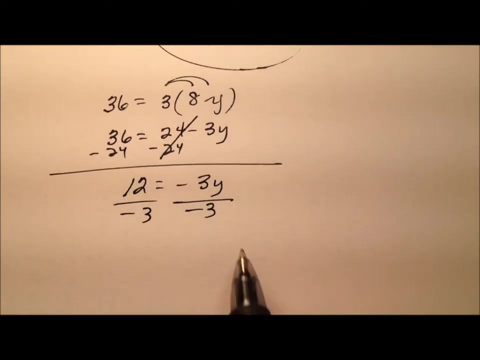 we need to distribute that 3.. So 36 equals 24 minus 3y. So if I subtract 24 from both sides, I'll get 12 equals negative 3y, And then let's divide both sides by negative 3.. 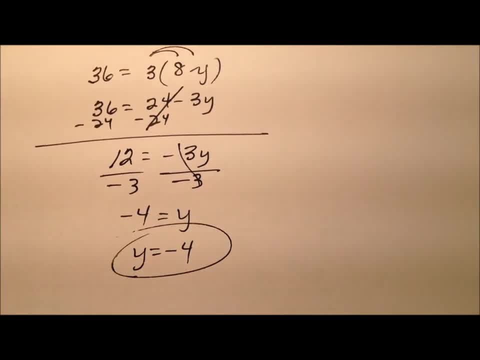 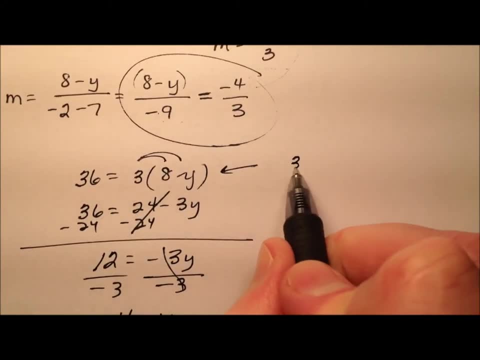 So that's what that y-coordinate is going to be. One note here on this equation: if we had, I'll just rewrite it here: If you didn't want to distribute, you could have just divided by 3, right then and there, And then you could have seen that 12 equals 8. 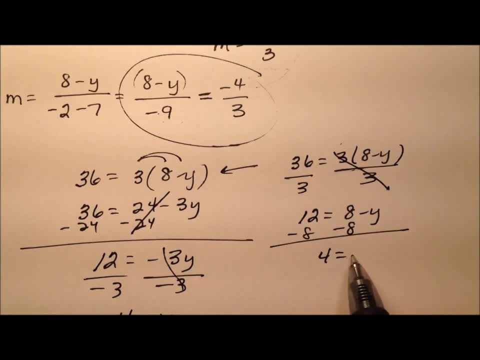 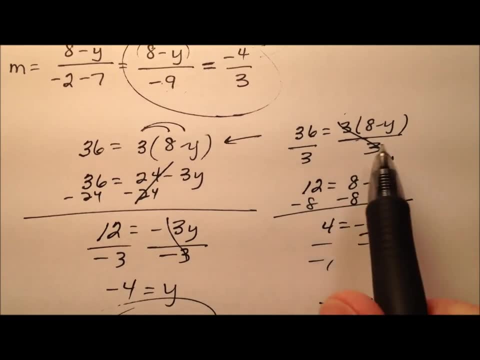 minus y, And then 4 equals negative y And y equals negative 4, just like we have there. So it's about the same amount of work in this case. But if you didn't want to distribute then you could have divided the 3 outright right there. And that's just a note about. 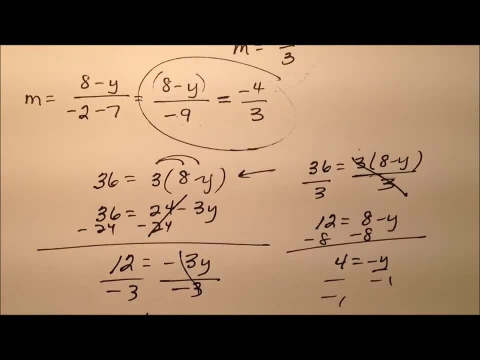 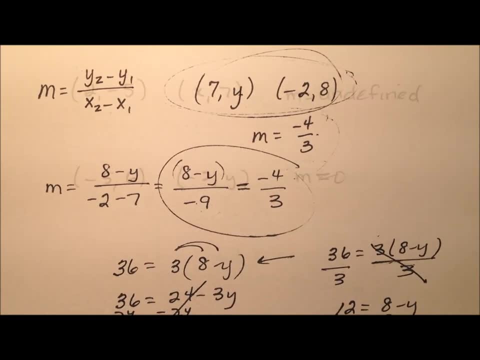 solving that equation. But we still have y equals negative 4 for this y-coordinate between these two ordered pairs, knowing that the slope was negative 4, 3rds. Well, I think I said at the beginning of the video we were going to work through two examples, But I 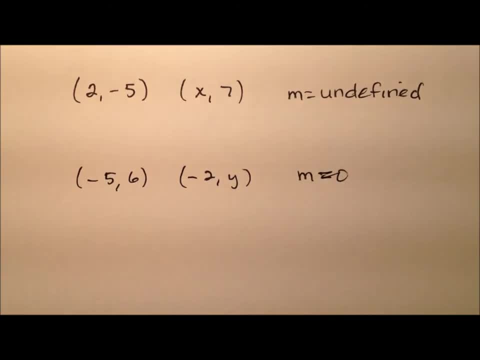 would be remiss if I didn't hit vertical and horizontal lines as well looking at these situations. So let's look at one of each real quick. So in a previous video, when we were talking about finding slope, we mentioned that if the slope is undefined, it's because it's. 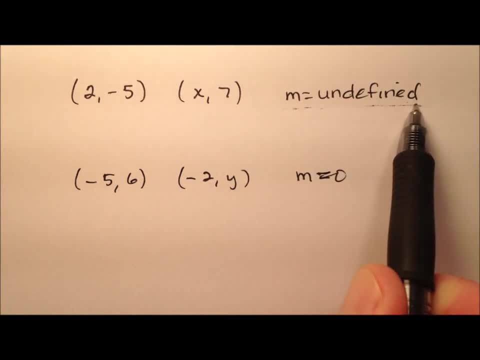 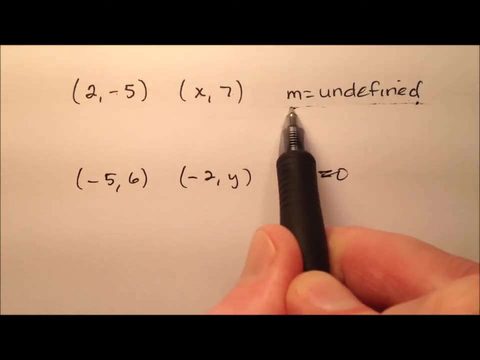 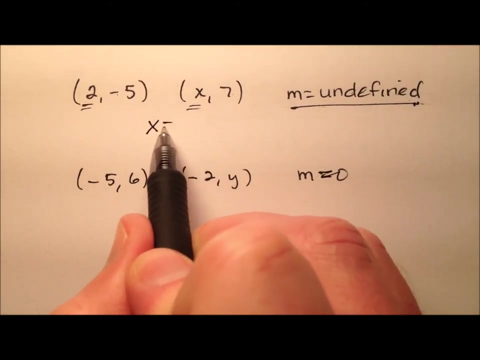 a vertical line and your x values were the same. So, looking at this, we have the ordered pair 2 negative 5 and the ordered pair x 7.. Well, in order to force the slope to be undefined, our x values had to be the same. So what is this x value? Well, it has to be 2.. OK, Like.